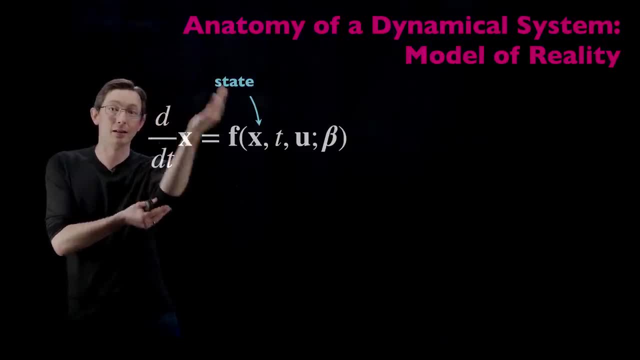 pendulum is uniquely defined not just by its angle, theta, but by its angular rate, theta dot. So the state of that pendulum system is defined by its angular rate, theta dot. So the state of that pendulum system is theta and theta dot in a vector. Okay, so that's what X is. X is a vector of the. 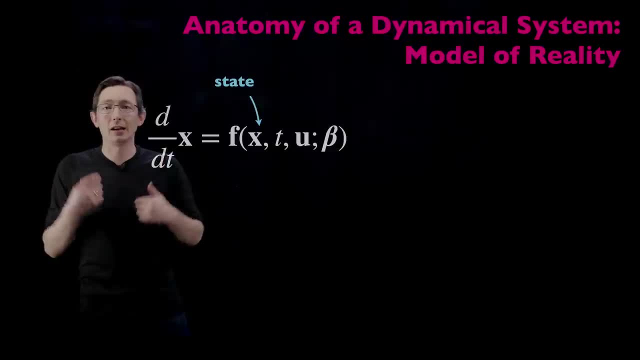 state of your system. If I'm looking at the stock market, the state of the system might be the value in all of the stocks and there might be more information that needs to go into that state vector. If I'm looking at the weather, it might be. 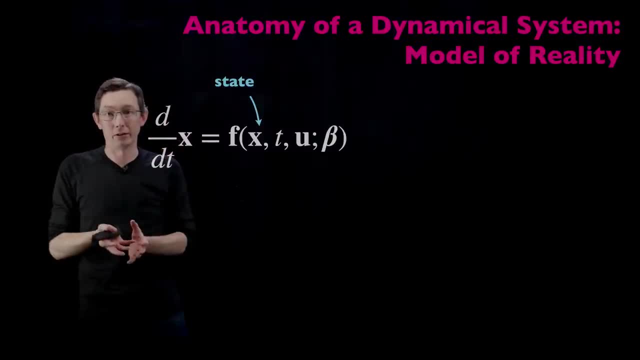 the weather condition on a one kilometer grid on planet Earth. Okay, so, the state vector X can get very, very large, but it's a unique, minimal description of the system you care about. Okay, F is what we call the dynamics. It's a set of functions: F1,, F2,, F3, that. 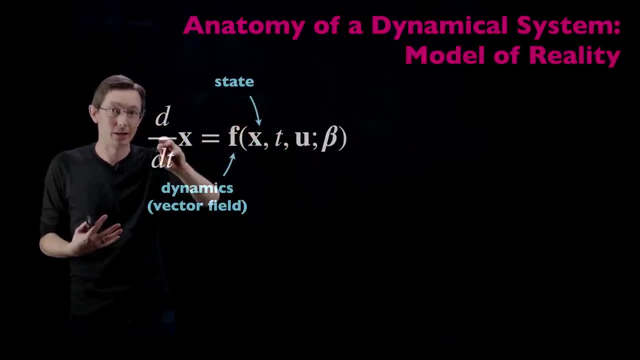 describe the dynamics of state 1, state 2, state 3.. So the time derivative of X1 will be given by the first row equation F1, and the time dynamics of X2 are given by F2, and so on and so forth. So F is a vector-valued function. that tells me. 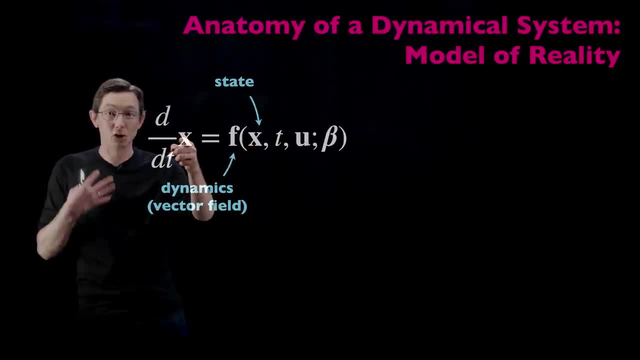 given a current state X, how does that state change in the next time instant? Okay, so that is the dynamics. It's a set of functions. Oftentimes this is given by, like Newton's second law or something like that, And we sometimes say that this is a vector field, because for every point in 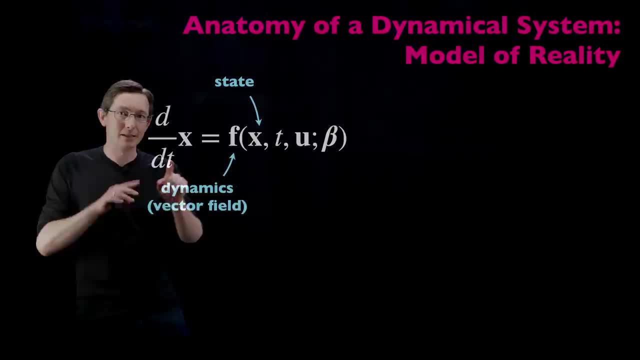 space X. this vector field essentially tells you how the derivative is pointing and what vector direction X dot is pointing at that point in space. So it's a field of these direction vectors. T is time. and this is really important for you because- think about it for a moment- because in lots of dynamical systems the 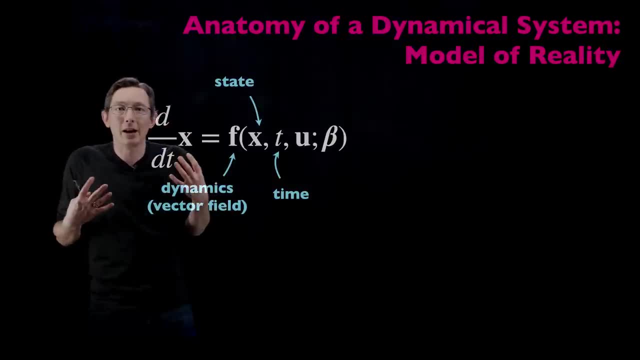 system itself changes in time. Okay, this is super important. Think about your brain state. Your brain state, the dynamics, the equations that would describe how your brain works, are fundamentally different when you're sitting here watching a video lecture versus when you're asleep. Different dynamics, Okay, so this is time. 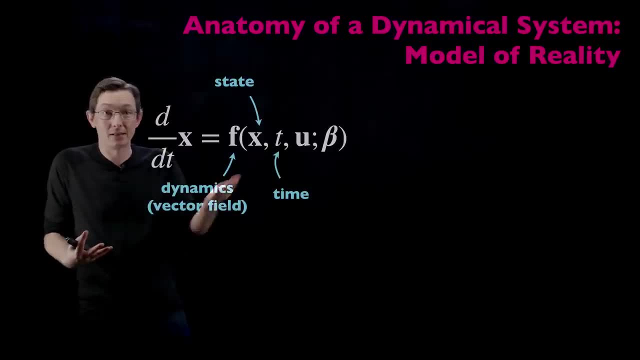 varying. The weather might change, The climate might change. Maybe we are actively changing the dynamics of a system dynamics. The vector field of the ocean changes in time. Good, U are all of the variables that we have active control over. So maybe we have some variables we can manipulate to. 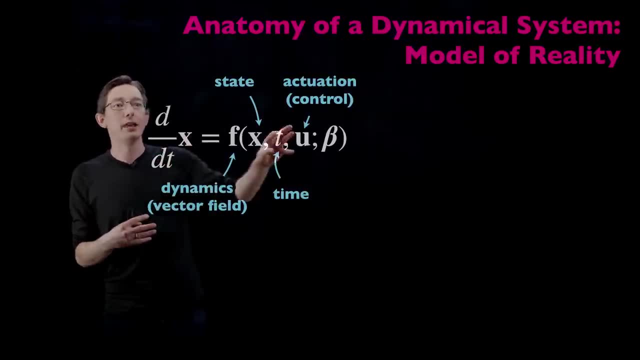 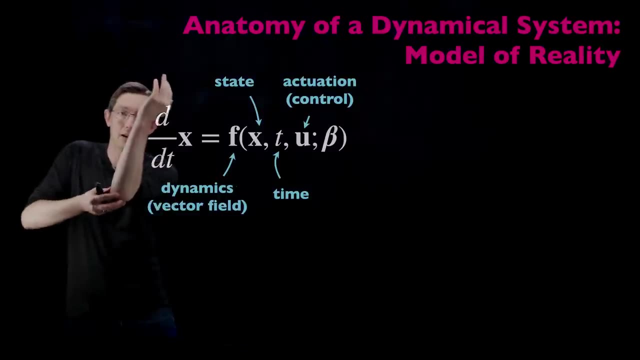 try to change the behavior of the system. Those are our control knobs and those go in this vector U. So in the case of the pendulum, maybe I put that pendulum on a cart and I can accelerate that cart, I can drive that cart around and that would be my control. 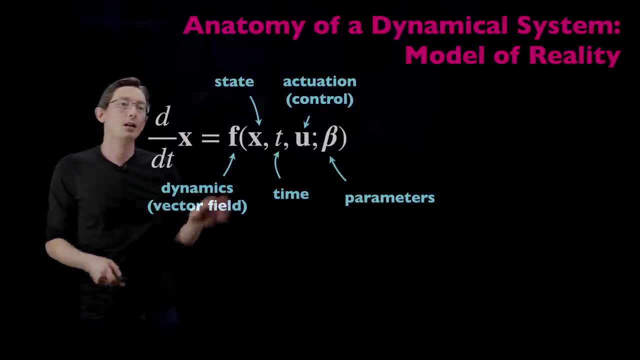 input U to try to change the dynamics of my system. Beta are all of the other parameters of the system that I don't explicitly have control over, but I might want to analyze and understand. So in the pendulum example this might be like the length of the pendulum. 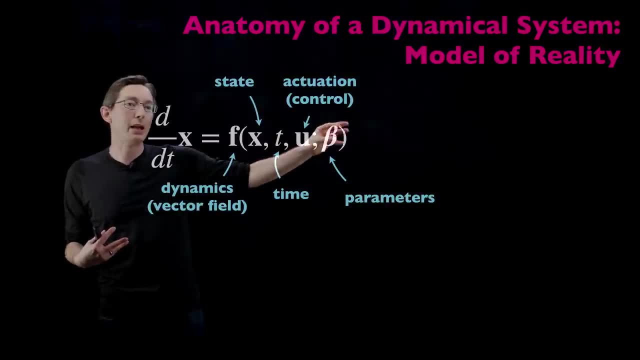 arm or the mass of the pendulum, things like that, And so these beta parameters. we want to understand the explicit dependence of these dynamics on those beta parameters. As I change those parameters I might get really big changes in the dynamics called bifurcations. 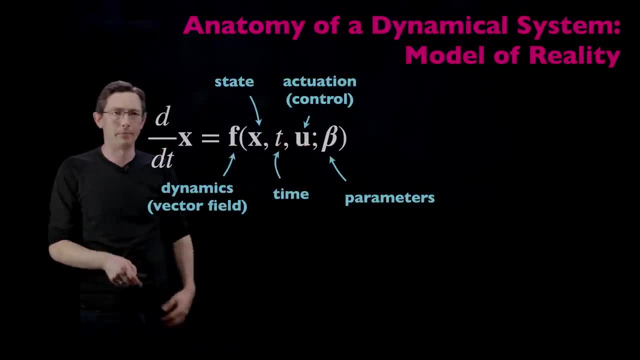 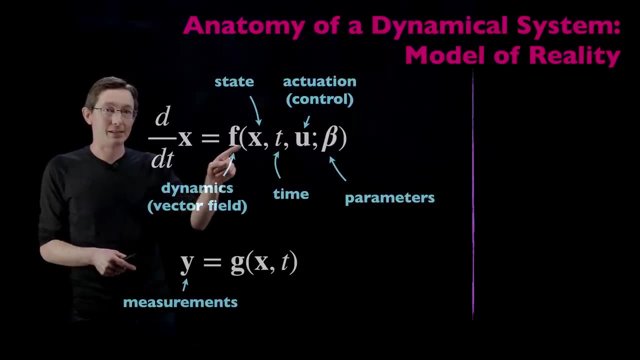 And so these beta parameters are super important. Good, So that's our dynamical system. Now, in addition, we also have measurements of our system, So we don't always have access to this full state X, because maybe my system is exceedingly large, You can't measure all. 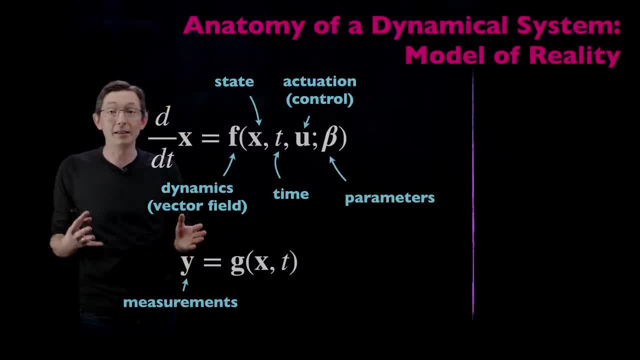 of the brain, all of the neurons in your brain. That would be completely impractical. So maybe you can measure a really, really small subset, or even some crude measurement, some proxy measurement like EKG or EEG or something like that. So you have these measurements in Y. And now that we've kind of talked about what is the 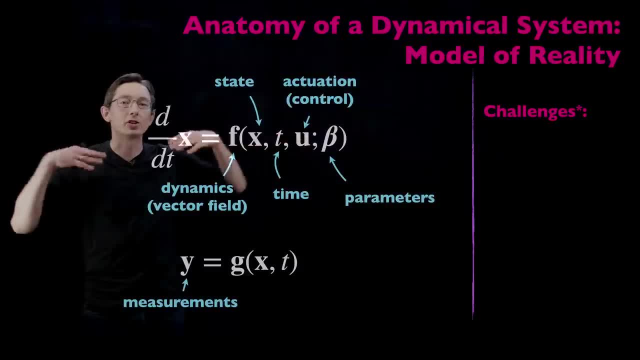 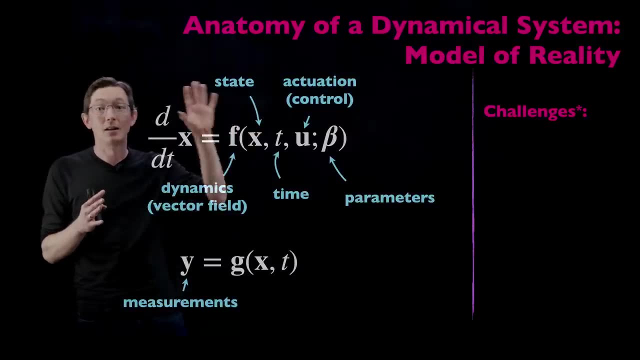 anatomy of a dynamical system. I want to walk you through what are the modern challenges. So people have been writing down dynamical systems and studying them and analyzing them for centuries. Newton's law, second law, is a dynamical system. That was kind of the beginning. 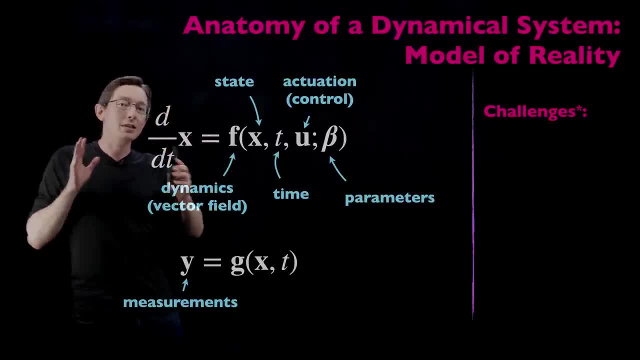 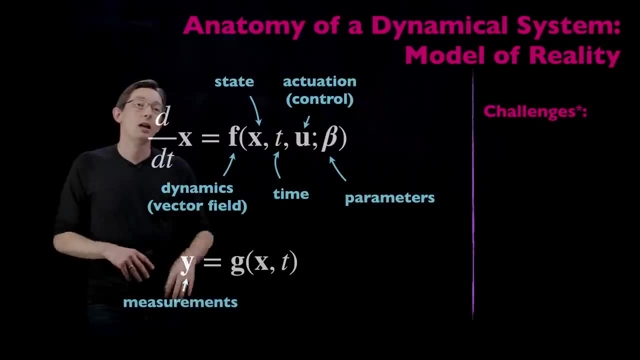 of our foray into dynamical systems. But in the modern era, a lot has changed and there are some big challenges that we're able to start tackling now, And so that's really what I want to talk about here. So in modern dynamical systems, some of the biggest challenges- probably the biggest one- 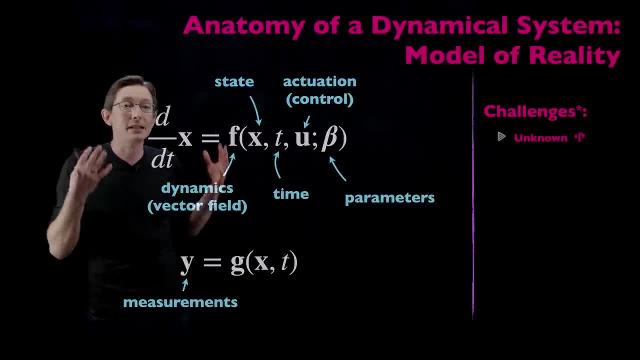 that goes unmentioned in a lot of cases is that in most situations we actually don't know F, We don't know the dynamics, We don't have a model of our system. So for mechanical systems like the pendulum, yes, you can derive Newton's laws, or the Lagrangian or the Hamiltonian. 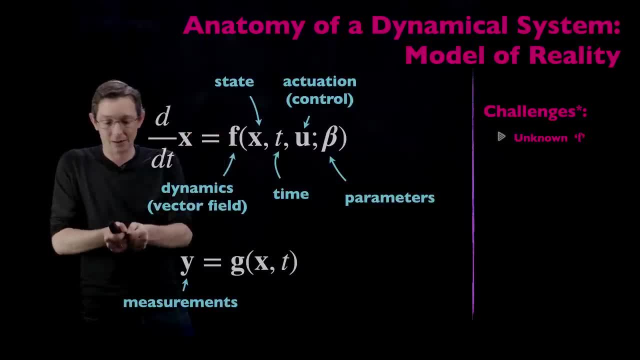 and you can derive these equations of motion from first principles. That's like you crack your physics book and you derive the system from scratch. That's how we, you know, used to do things. That's how we do things when we can. 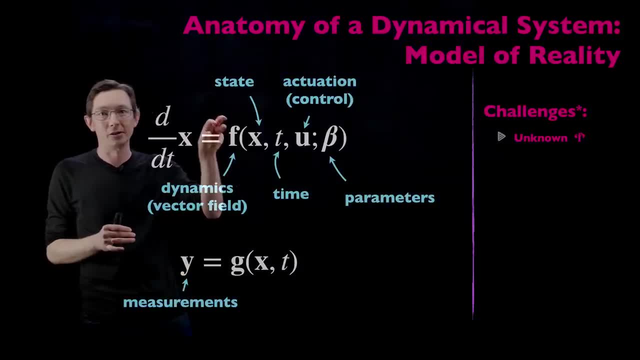 But for modern systems of interest. we don't have access to these governing equations in F. There is no known master equation for how your brain works. We don't know the F for a brain. We don't know the F for a disease network. We have models, We have approximations. 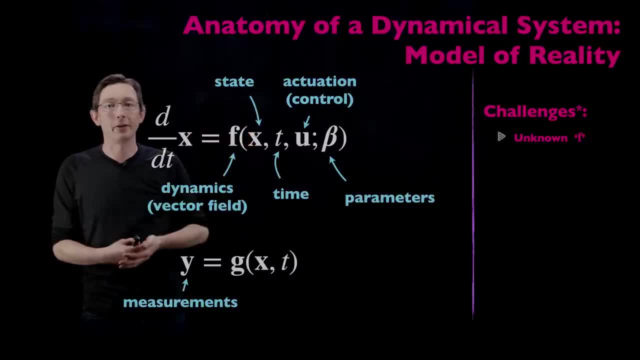 But we can't agree on one governing physical law for how a disease spreads or how the climate works. Okay, So modern systems of interest. F is often unknown. Even in systems where you do know F, like the Navier-Stokes equations for a fluid, it might be far too complicated. 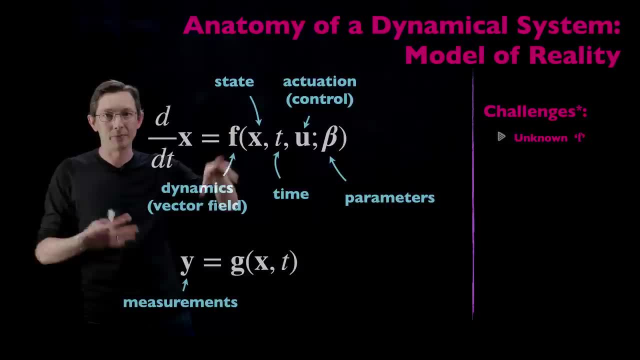 to use, and so we would need to learn a reduced order model in terms of the things we care about, in terms of a less descriptive state X that captures the big things I care about in my fluid. The other really really big challenge in dynamical systems, and I think 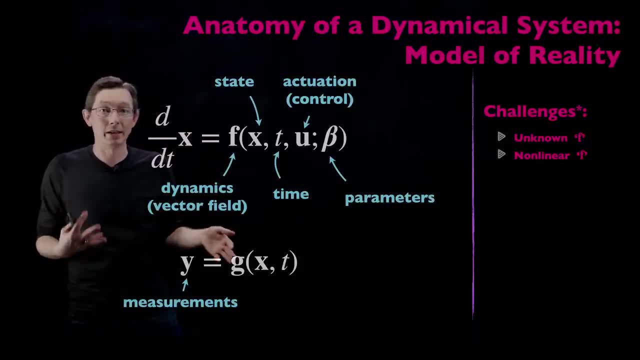 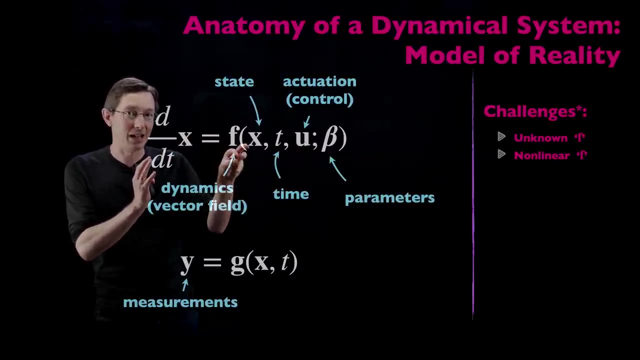 this one is really important. Okay, It may be tied, for number one is non-linearity. So this function F in general for systems of interest is often non-linear And that means superposition of solutions doesn't hold. If my dynamics were linear, if X dot equaled a matrix A times X, everything would be simple. 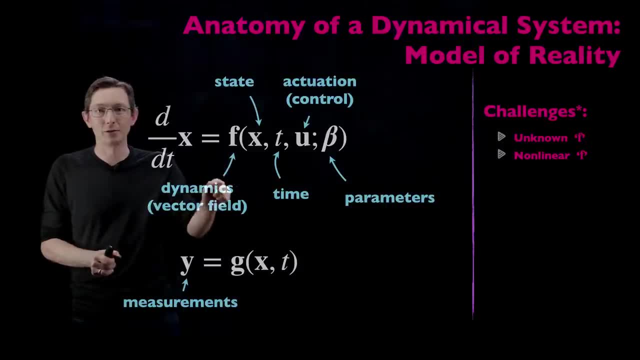 There would be a canonical closed form solution. You could just write down the solution and go home. We would all be out of business. So non-linearity is what gives us job security in dynamical systems. This is the. The real challenge in many systems is that even small amounts of non-linearity make it. 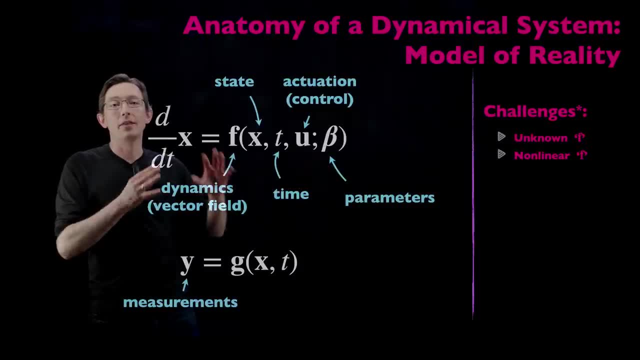 so there are not closed form solutions. in general, There are special classes of non-linear systems and special solutions that you can find, but there is no generic one-size-fits-all non-linear theory of non-linear dynamical systems. So that's really interesting And 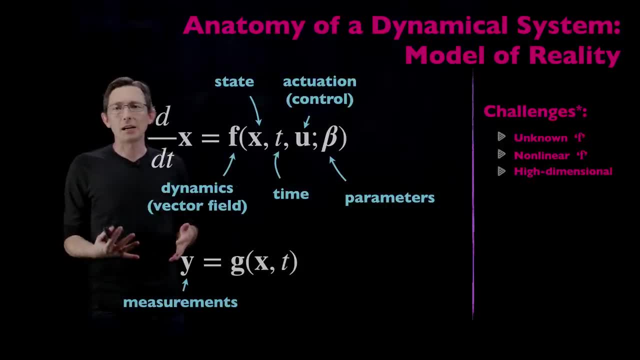 most systems we care about are non-linear. Other challenges are dimensionality of the state vector X. Okay, So for many, many systems, this state vector X might be exceedingly complex. I think in your brain there are estimates that you have 100 billion neurons, That's 100 billion dimensional. 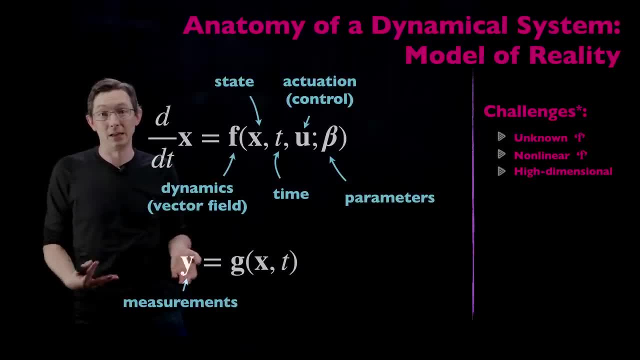 state vector just to describe the state of all of those neurons. uniquely Describing the climate or the weather is also very, very massive problem. If you want to get a really good description of weather on planet Earth, you need a very high resolution and Earth. 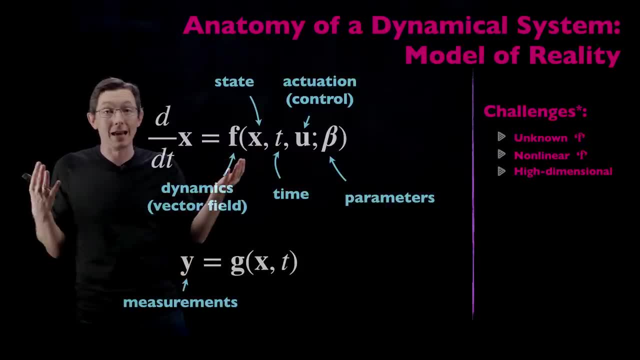 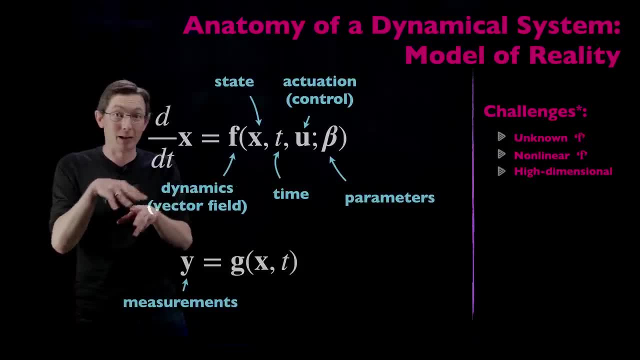 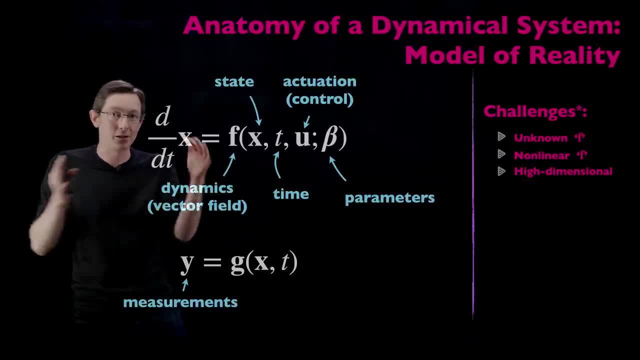 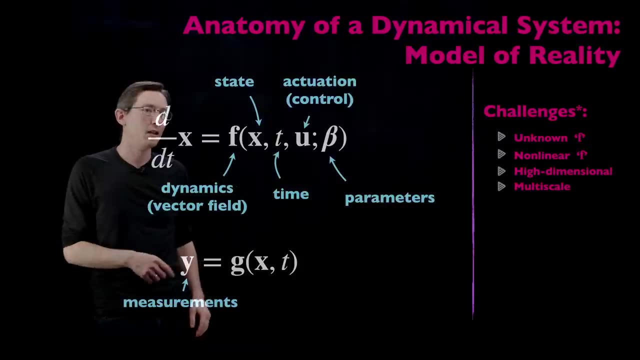 interact And that's you know, there's billions of us and there's tons of connections in this network. So it's super complicated, high-dimensional dynamics in a lot of cases and that makes it really hard to analyze. these Along with dimensionality is multi-scale, So these dynamical. 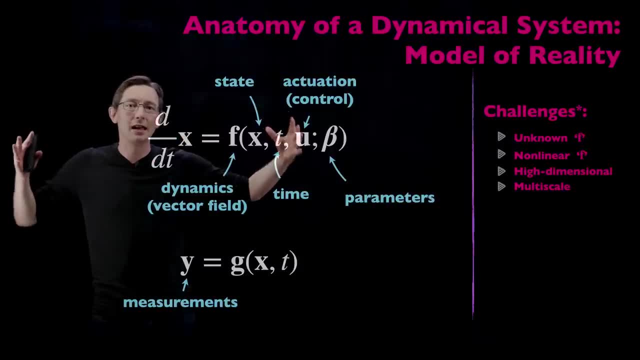 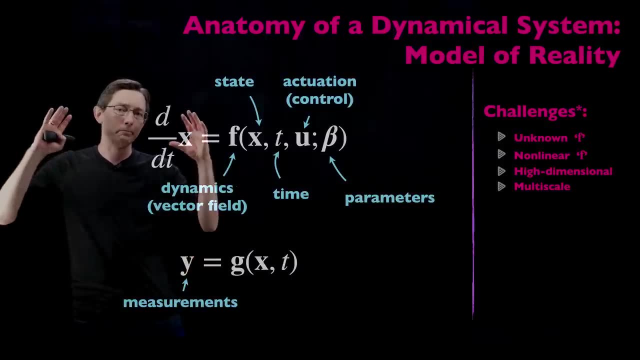 systems are not just big, but there's a range of scales from, you know, big scales all the way to really really small scales. So think about weather or climate, You know, on the scale of the size of Earth. there are things I care about. There are seasonal. 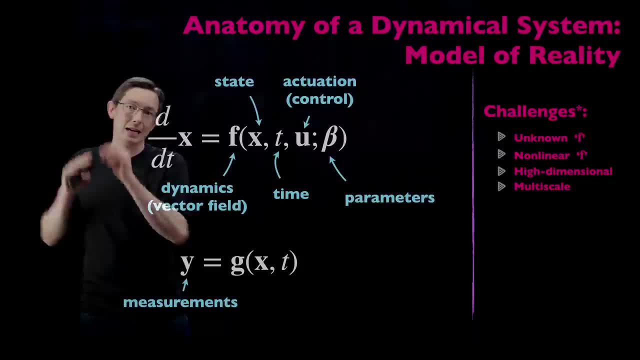 changes. you know big hurricanes, But little, teeny, tiny features also might matter for the weather prediction three weeks out. Okay, So you have this range of scales you care about. Your brain also is fundamentally multi-scale. spatially, There's regions and then those. 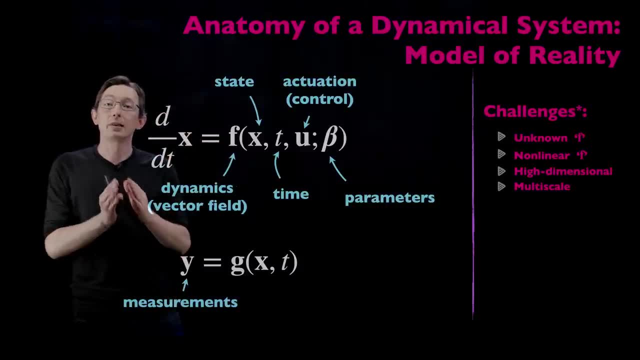 regions are composed of, you know, individual neurons and things, But there's also multi-scale in time. You're listening to me talk about this right now. You're hearing words on a time saying on seconds. You're connecting that to things I told you a few minutes ago. 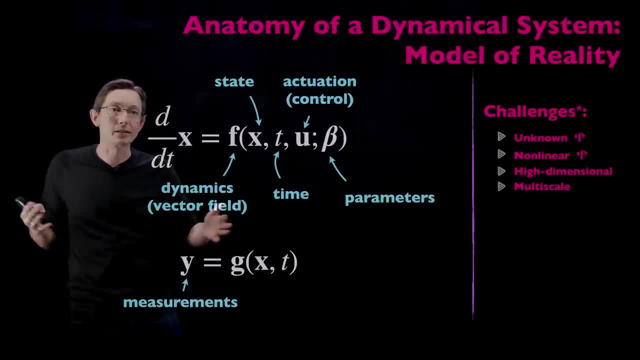 But you also have this lifetime of experience over months and years, So you're extremely multi-scale in time. Dynamical systems are fundamentally chaotic in a lot of situations. So not all nonlinear systems are chaotic, but many of them are, And what that means. 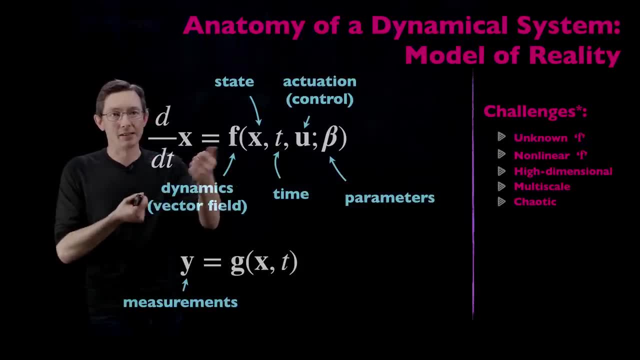 is that you get a very sensitive dependence of the outcome of these systems. The future depends very strongly on systems, On small changes on the initial condition and the parameters and the dynamics now. So if you have your system and you change your parameter, even by a little bit, you might. 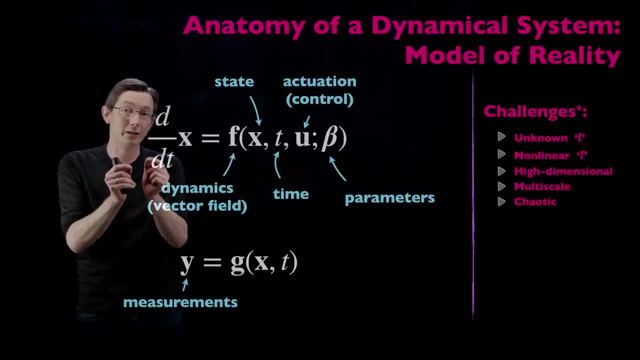 get very, very different phenomena, Or if you change your initial condition a little bit, you might go to very different places, And that makes it really hard to predict these systems. So that's actually why weather is so hard to predict. You know, we can't predict. 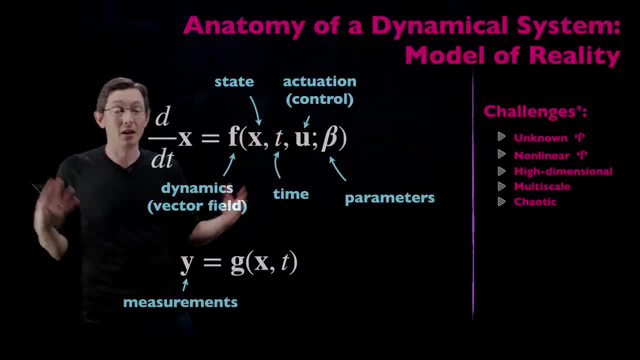 three weeks out, because this is a super chaotic system and we can only measure the system so accurately and we only can describe the outcome. So chaos is still a huge problem. Latent variables, hidden variables- again, this is related to dimensionality. If I have a big state vector, chances are I'm not measuring everything. 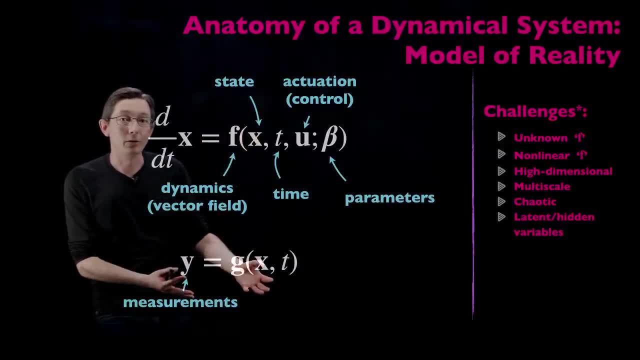 You can't measure all of the neurons in your brain. You might only measure a few of them. You might only have a proxy measurement. So latent variables, hidden variables, is a big deal. They might matter a lot and you can't measure them. What do you do in those situations? 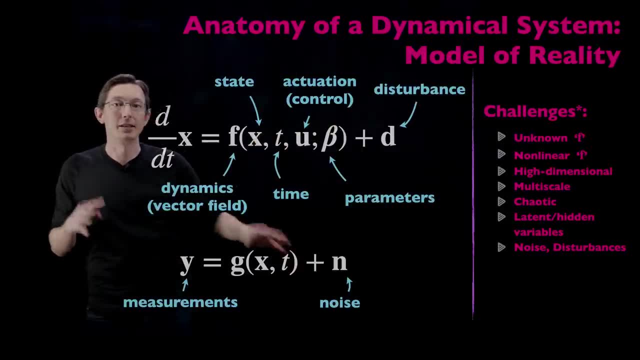 All real dynamical systems are very, very complex. They're very, very complex And you have to consider this. So your dynamical system is going to be forced by external disturbances, stochastic forcing, and your measurements are going to have noise, And you can't always. 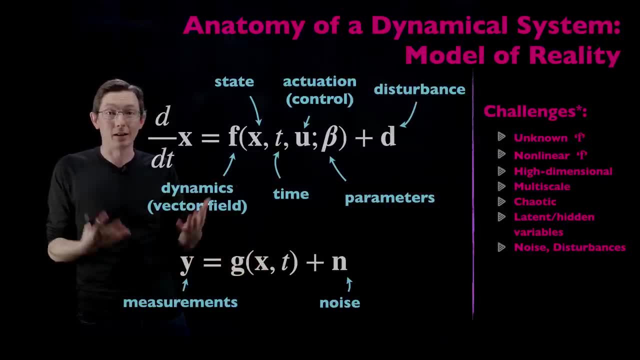 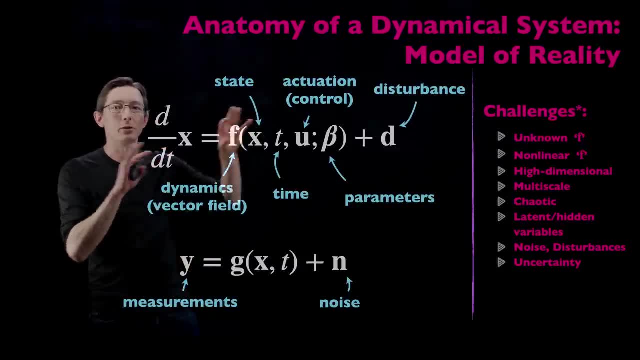 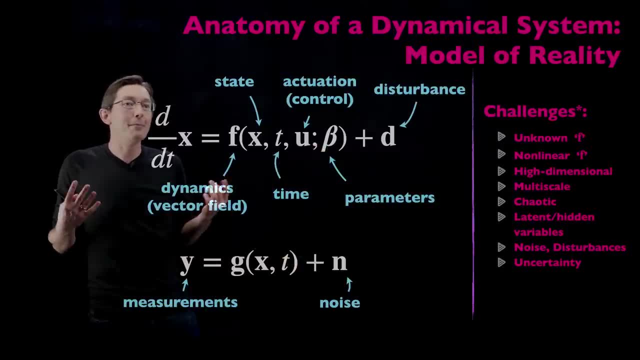 uncertainty in what I'm measuring and how it's being measured. I might even have uncertainty in the measurement time of when I take that measurement. I mean, there's all kinds of uncertainty and that all will kind of conspire to make this a very challenging problem. Okay, And I have an answer. Okay, Okay, Thank you, Yvonne. Thanks guys. I have a question. I just want to know, you know, a question that I've heard all day about neural networks: What kind of natural world does the human spirit live in, Or does it just kind of live in a normal world? 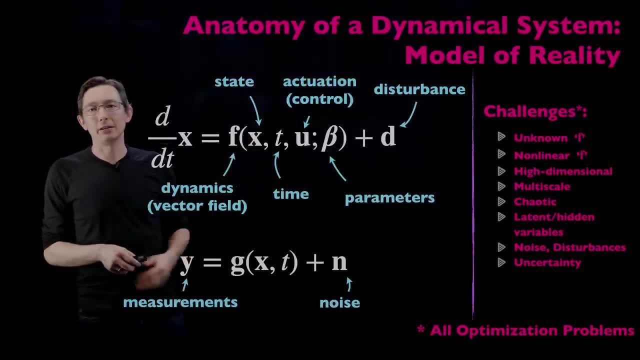 Okay, And I have an asterisk on the challenges because I want to point out that most, maybe not all, but most of these problems can be recast as optimization problems, So kind of optimally handling noise and disturbances for future predictions or estimation optimally propagating. 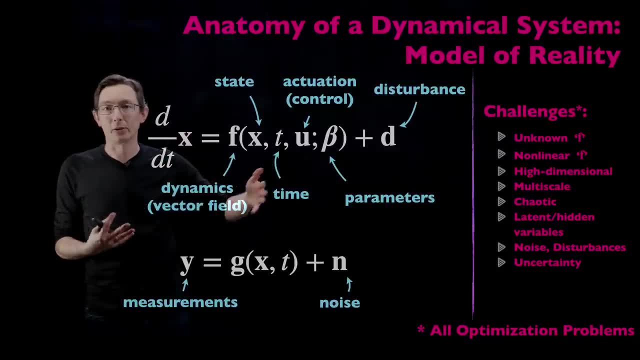 uncertainty in the future, and so on and so forth. Optimally reconstructing the full state from limited measurements. Why And when I say that this is an optimization problem, you should be thinking. now I can probably start using tools from machine learning, Because machine learning. 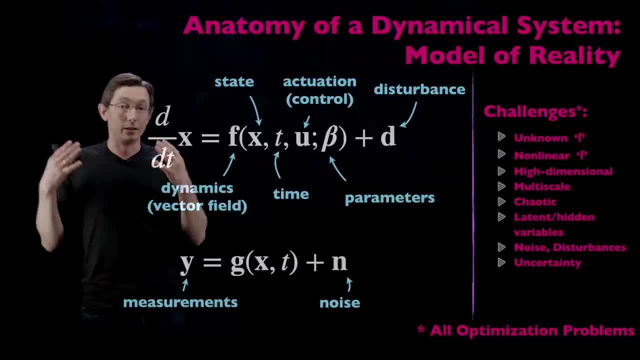 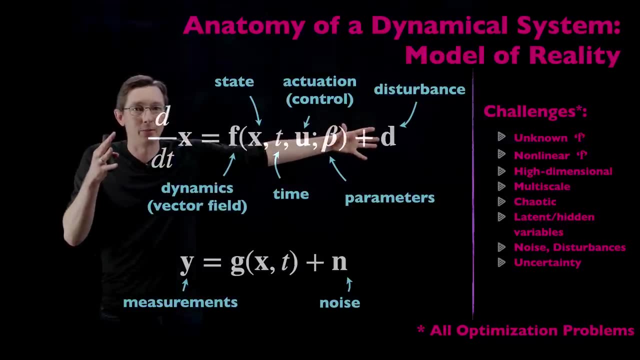 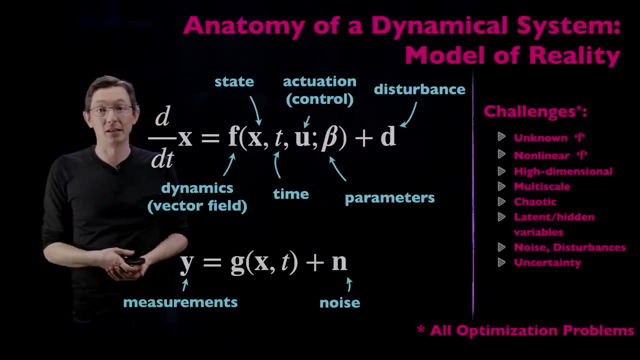 is just optimization based on data. It's building models using optimization and a wealth of data, And so this is really nice because modern dynamical systems- kind of the anatomy of a dynamical system- allows you to focus on individual tasks and challenges with these emerging optimization. 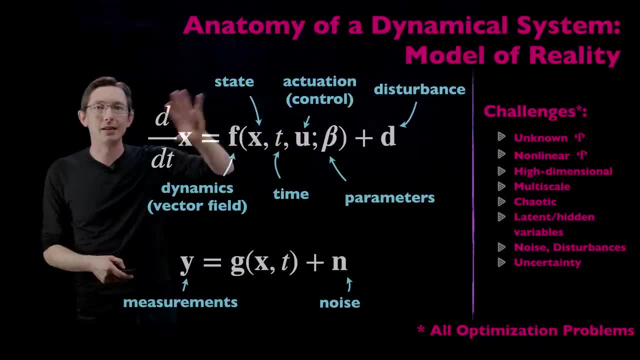 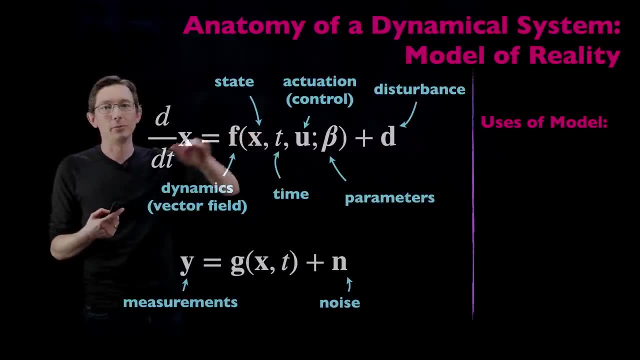 techniques, Okay, Good. So now that we've understood kind of the anatomy of this dynamical system, I want to talk a little bit about how we would use it. And there's so many uses. I'm just going to briefly, briefly touch on some of them. Of course, we might want to predict the future state of the system. 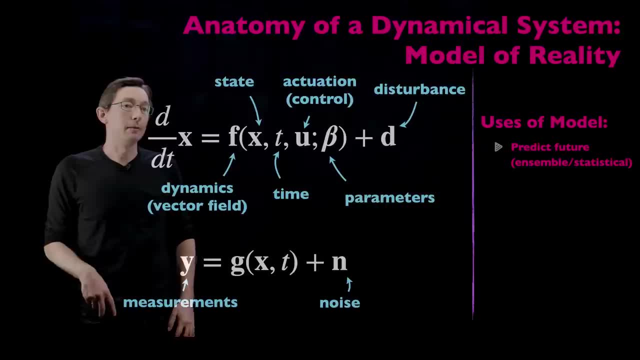 So I might want to predict the weather a week from now. When I think of future state prediction, I think of what if someone's lost at sea? Okay, So we had some rough idea of their initial condition and we want to integrate where we think they'll be two hours later. Okay, So that's a future. 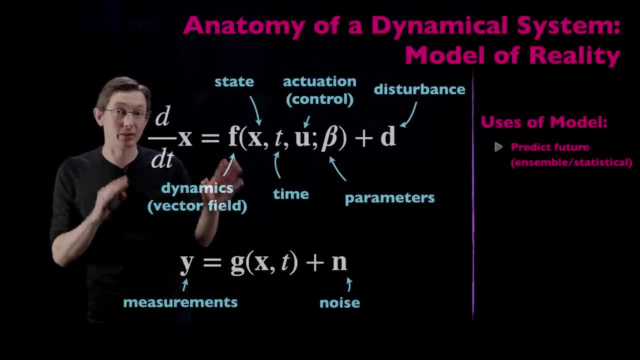 prediction, And the future prediction doesn't have to be deterministic, It might be statistical. I might have to run an ensemble of initial conditions. Maybe I have uncertainty of where that person was lost at sea, Or maybe this is the Gulf oil spill and I don't know exactly where the oil 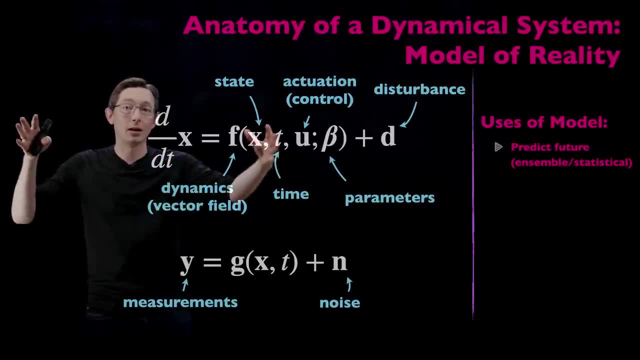 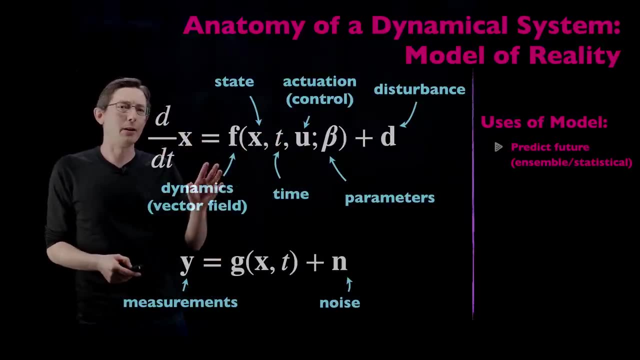 is coming up. So I have a Gaussian of uncertainty and I want to propagate that into a future estimate of where the distribution of oil will be. So that's a statistical or an ensemble prediction, And I'll point out all of these topics every term in this dynamical system. every one of those. 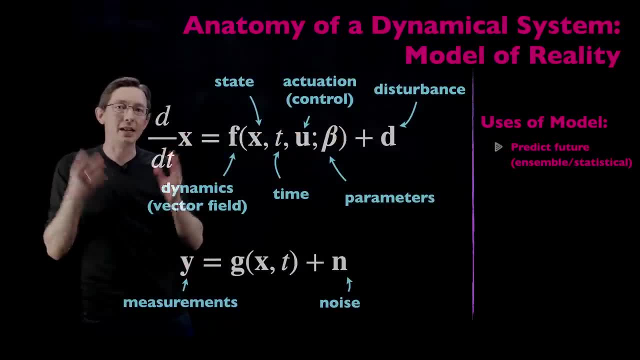 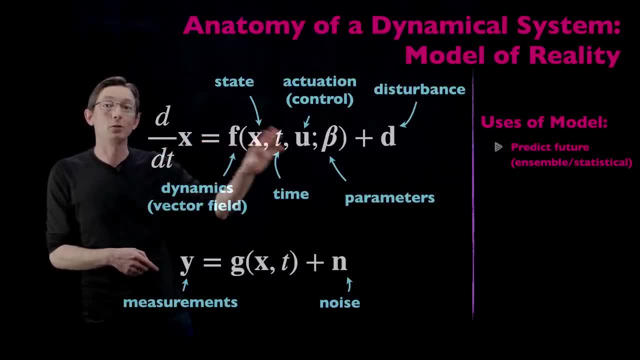 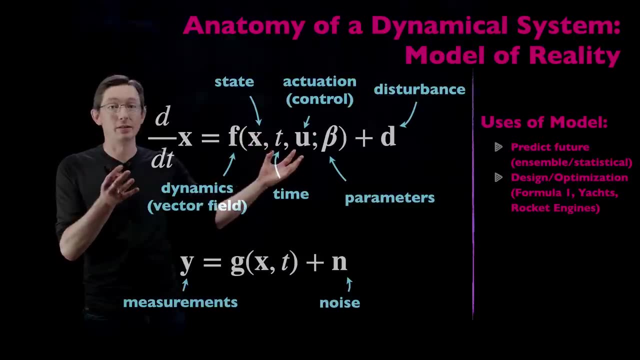 on these problems. These are not challenges, These are whole careers. Okay, Design optimization: that's another big use of dynamical systems models. What I might want to do is, now that I have a model of my system, I might want to design betas to get a performance or an output that is. 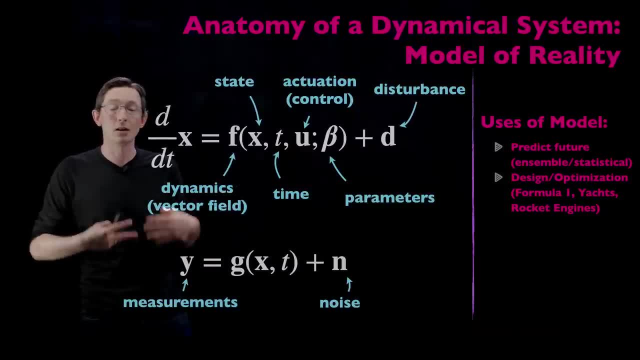 desirable, So think Formula One cars or super yachts or rocket engines. I want to design the parameters of my system to get some desired high level output like drag and lift and things like that. Okay, And so that requires you to be able to understand how your system depends on these parameters. 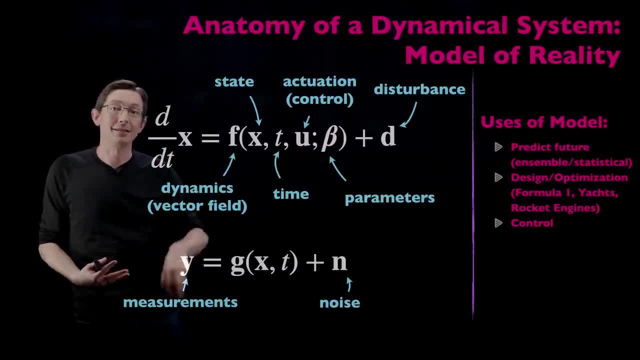 Now, if you do that optimization in real time based on your measurements, that would be called feedback control. So if you can actively manipulate some part of your system in real time, those parameters become actuators and this becomes a feedback control problem, And that would be really satisfying and incredibly useful. 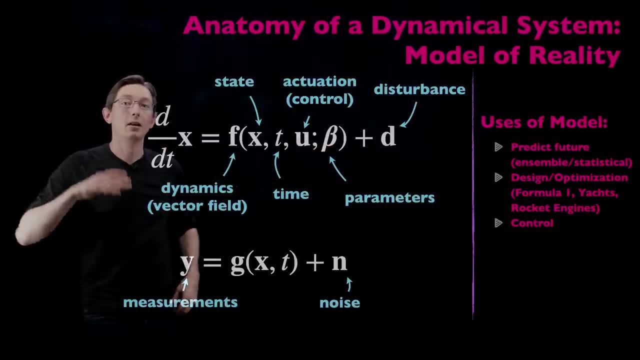 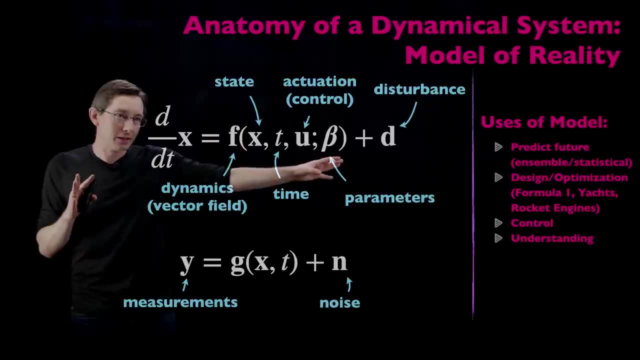 in many, many systems if we could actively control them. to some engineering, you know specifications. Now, most of the first uses are very practical, very engineering oriented, but we also, as humans, deeply care about understanding the world around us. We don't just want to manipulate. 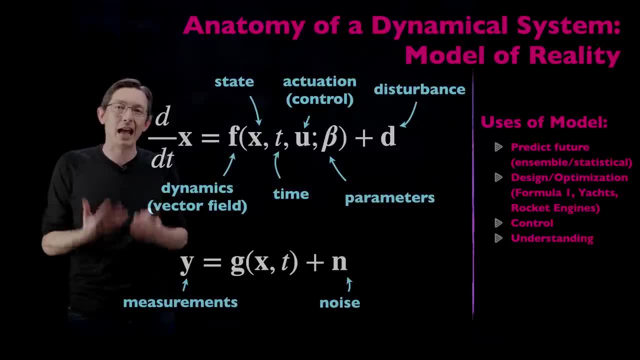 it. We don't just want to predict it, We want to understand fundamentally how and why it works. Okay, And these dynamical systems give you a very kind of intuitive way of understanding how the world evolves and what are the rules for how that evolves. 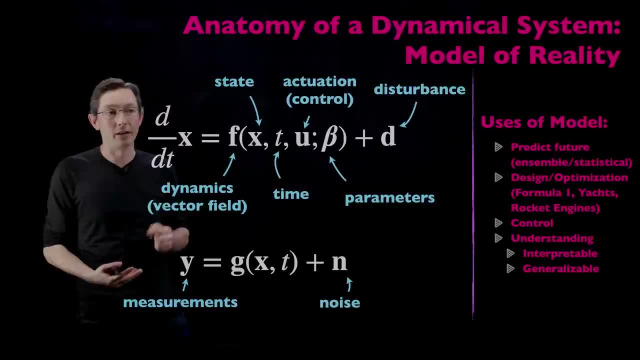 And so there's a couple of kind of keywords here that I think are really important: Interpretable and generalizable. So interpretable means that this model is not so complex that I can't communicate with you about it. If this model is not too complicated, we can talk about it. We. 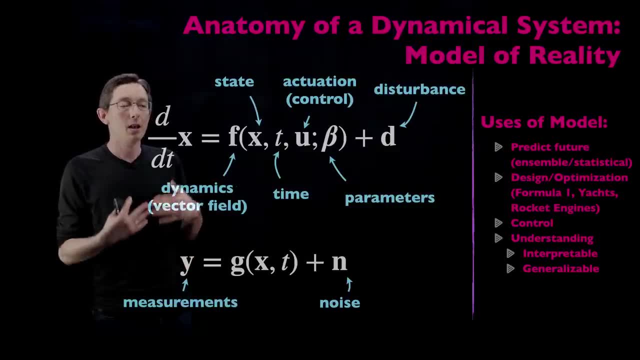 can try to understand it, We can communicate and interpret this model. Generalizable is also really important. If I write down this model, I want it to be useful in other scenarios. then I might not have thought of So being, you know, having some generality in how it. 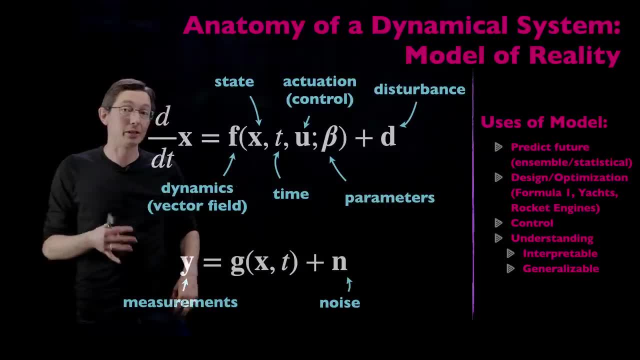 how this model works, even for parameters. I haven't tested. that's really important And I always think of Newton's second law as kind of the ultimate interpretable and generalizable dynamical systems. model F equals MA. It's super simple so we can interpret and understand it. 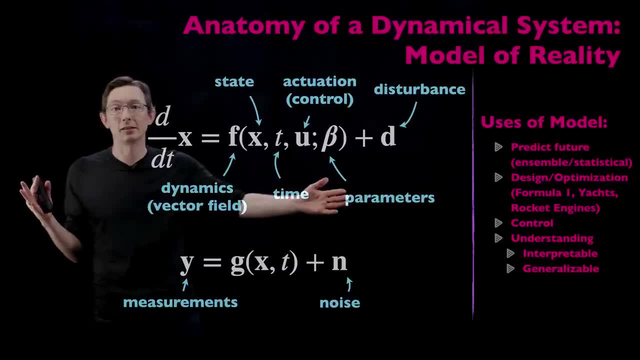 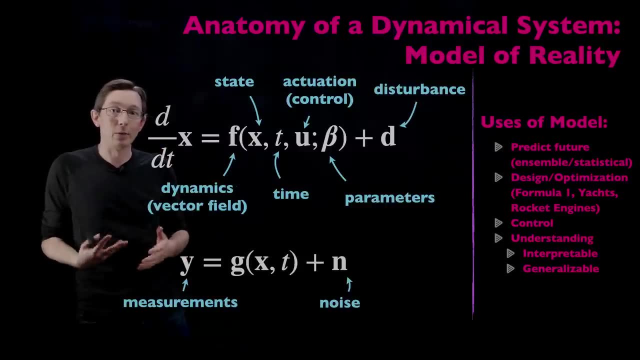 It is very generalizable, It works in so many scenarios, you know, for different parameters, for different state vectors and so on, And it fundamentally has, you know, a lot of things that we need to understand And it fundamentally has changed the way that we